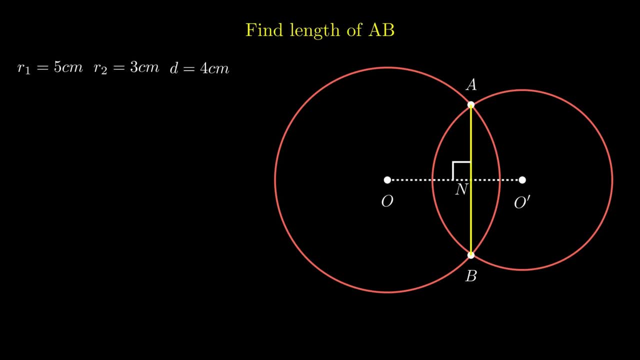 with reference to the circles with center O. By the application of the theorem, any line perpendicular from the center to the code bisects the code. So we conclude: segment A is equal to segment B. Therefore segment A is twice of segment A. 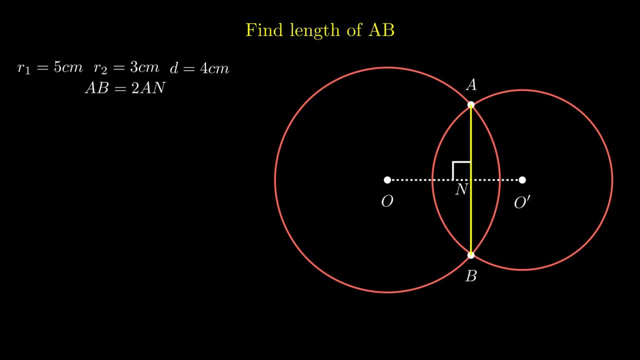 by using this angle, this equation- we will focus on segment AN to calculate the length of segment AB. Now, to find the length of segment AN, point O and point A are joined, resulting in the formation of a right angle triangle, AON, By using Pythagoras theorem, that is, in a right 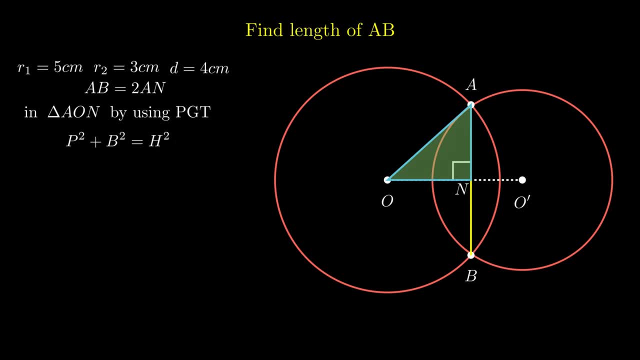 angle triangle, the sum of the square of the base and perpendicular is always equal to the square of the hypotenuse. On substituting the corresponding values of hypotenuse, base and perpendicular, we get ON square plus AN square equal to 5 square. Since this equation 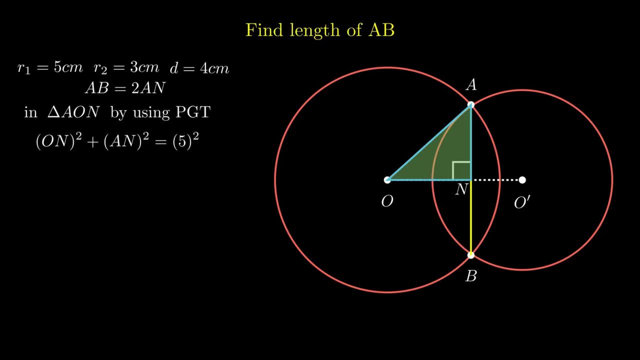 can't be simplified, as variable ON and AN are different. the solution to this problem is to have another equation with the same variables. In case you don't know how to solve such equations, please press I button on the top right of your screen. 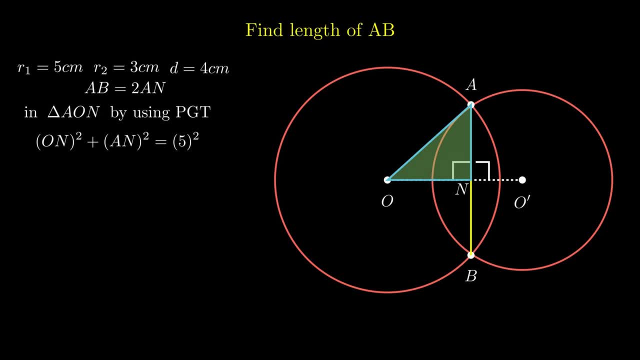 To form another equation with variable AN, consider right angle triangle AO-N. By using PGT again, O-N square plus AN square equals 3 square. On subtracting equation 1 and 2, we get ON square minus O-N square plus 0, equal to 25 minus 9.. Therefore, ON square minus O-N. 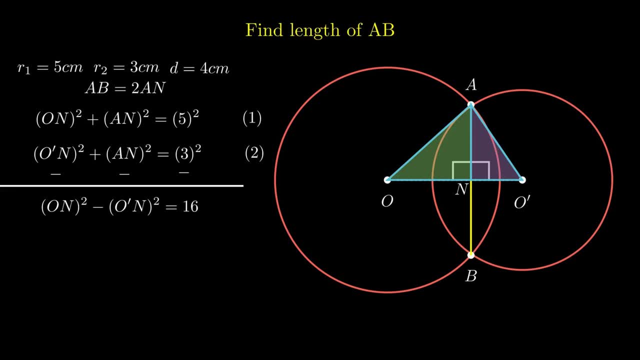 square equals 16.. Again, this equation can't be simplified further, as segment ON and O-N are different. The solution to this problem is now substitution, As there exists a relationship between O-N square and O-N square From figure segment ON and segment O-N square, segment OO', which 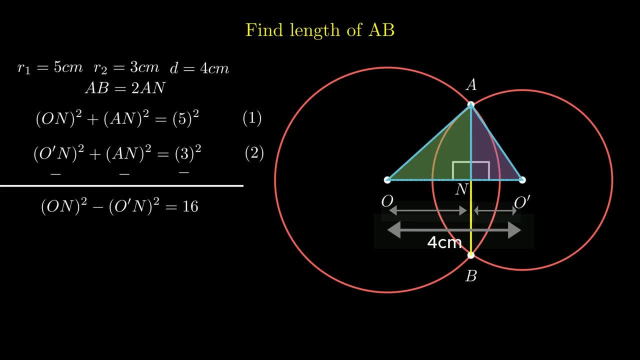 is equal to 4 cm. So if we assume segment ON equals X, segment O-N becomes 4 minus X. If we assume segment ON equals X, segment O' becomes 4 minus X. Now our equation can be simplified as both segments are expressed in the same variable. But if there would have